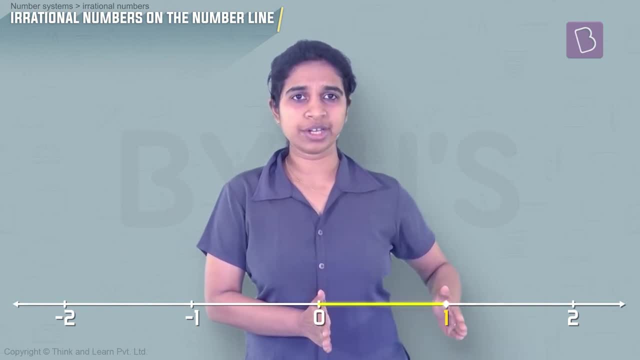 simplest way to plot it is from zero. I'll take one unit here, one unit this side, on the positive side of the number line, and one unit on top right. So I have one unit here and one unit on top. Now, what will the length of this diagonal be? Root two, simply because of Pythagoras theorem. 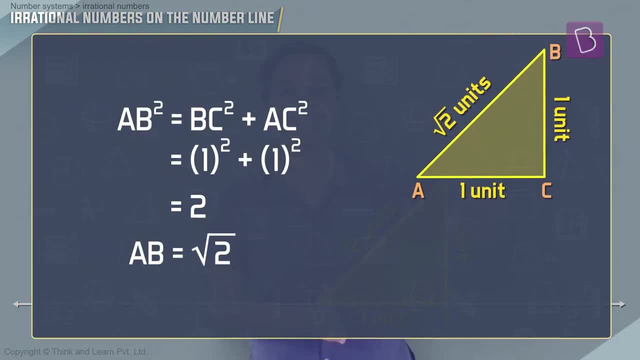 because if you look at this triangle, in this triangle one side is one, the other side is one right. So the third side, or the hypotenuse, will be nothing but square root of one plus one, which is why root two, correct, Which is why the hypotenuse is root two. Now just take a compass. 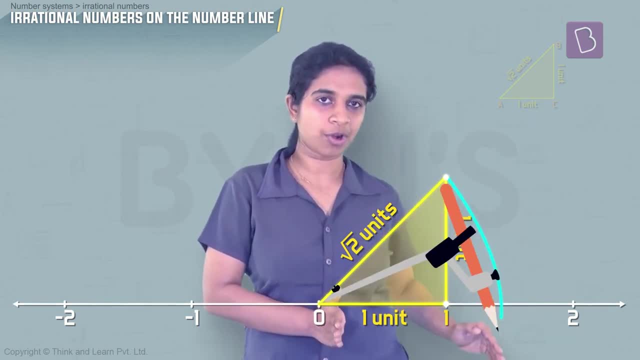 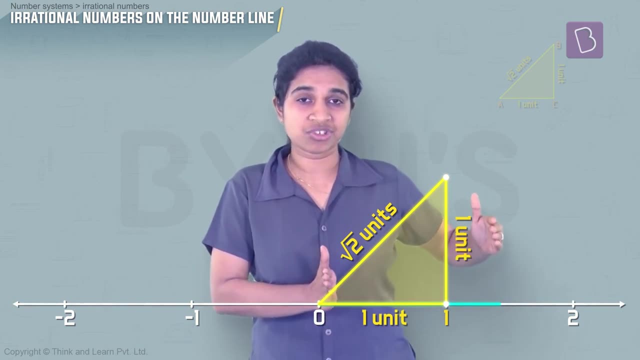 right. Keep it on the origin. the other end on hypotenuse and plot the hypotenuse right. Keep the radius constant, plot the hypotenuse on the number line, So you have your hypotenuse. the hypotenuse is nothing but root two. That means this distance is right. That's how you'll. 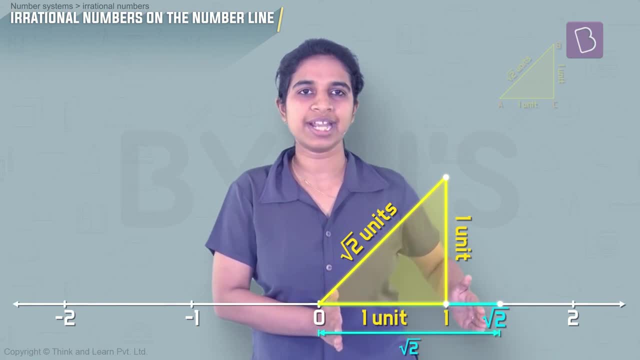 plot root two on a number line Simple using Pythagoras theorem: right, This side is one, this side is one. This is as simple as that, right? So you have root two now plotted on the number. Let's say you now want to plot root three. How would you do that for root three? Look at this. 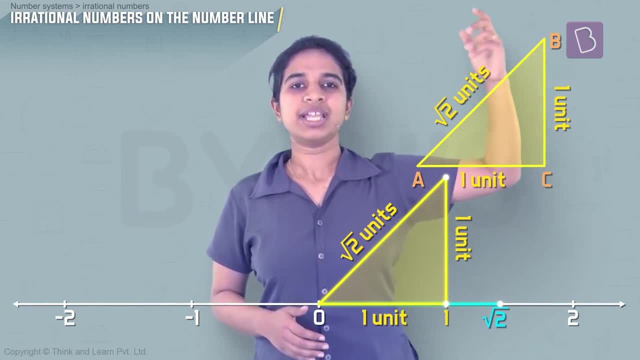 triangle again right, We had one plus one, We got two. If we want three, how will we get two plus one? Give us three right. And two is nothing but root, two square right. So in the same triangle. 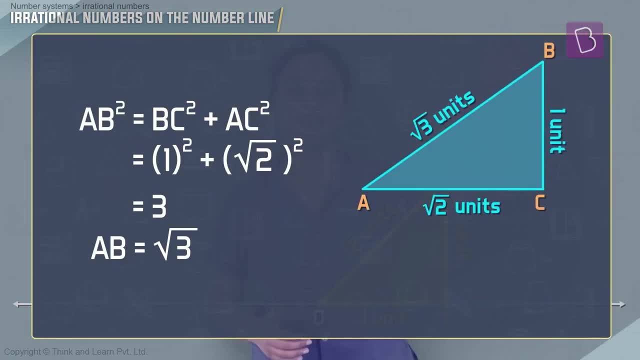 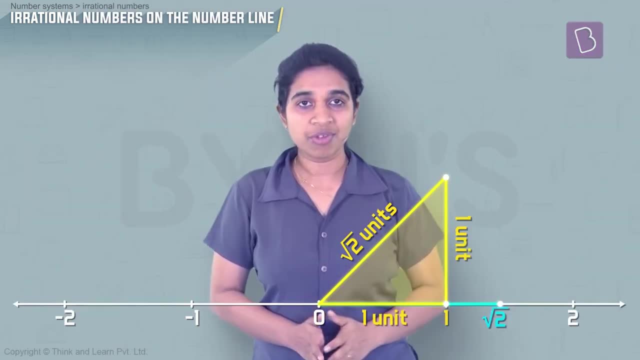 if I change this side to root two and keep this side as one, then my hypotenuse will be three right, Because root two squared is two plus one squared is one will give you three right. Now we've already plotted root two on the number line. Let's use the same root two, So you have root two. 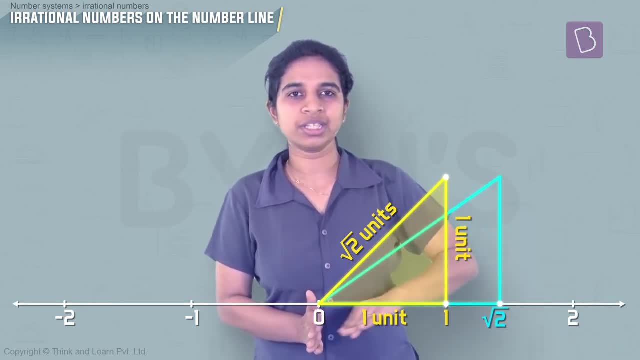 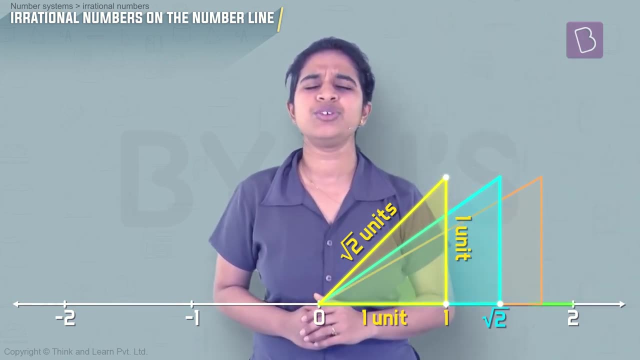 draw one from here. So you have a triangle. one side, root two, the other side, one. the hypotenuse of this triangle is going to be root three. right, That's how you get root three. Now you can go on and on, and on and you can plot the root of any number. So that's the way you will plot square. 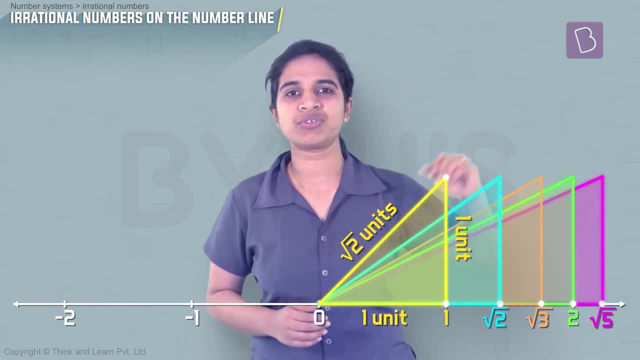 roots on a number line. right, We can have root four, root five, root six, and so on. right, Root four is any way too. It's easy. So all irrational numbers which are square roots, you can plot this.